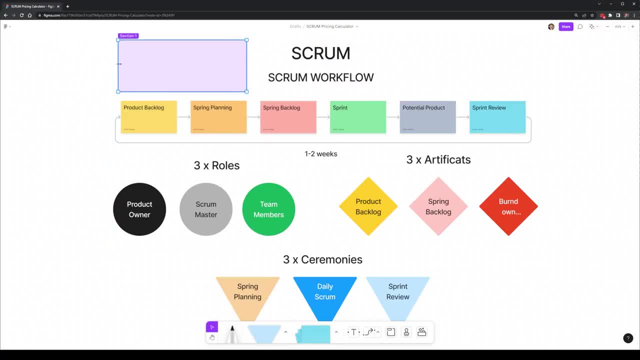 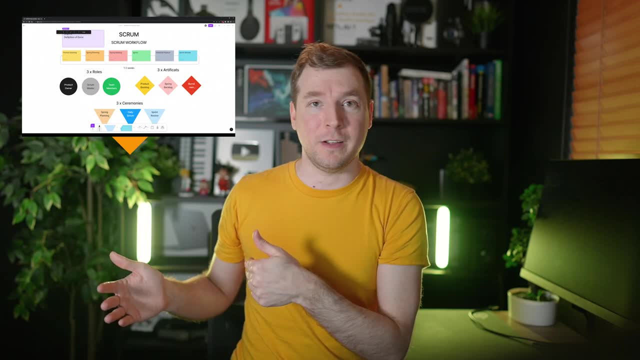 is, We'll go through the whole Scrum workflow, including all the main parts of it, such as the roles and artifacts and ceremonies, and how an entire sprint looks like and how to run sprints as well. Then, after that, we'll implement it with a project that I'm using, So you can see what it looks like. 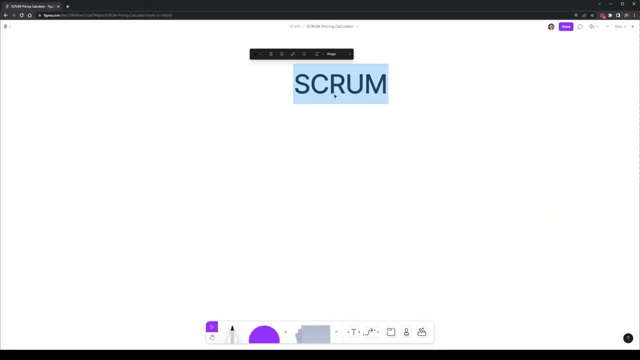 in practice. I'm creating a Figma board here, which you guys will have access to, which I'll be using as part of this Scrum demonstration, And what we're going to do is create a Scrum workflow. This workflow are the core aspects to create your own Scrum, if that's what you're. 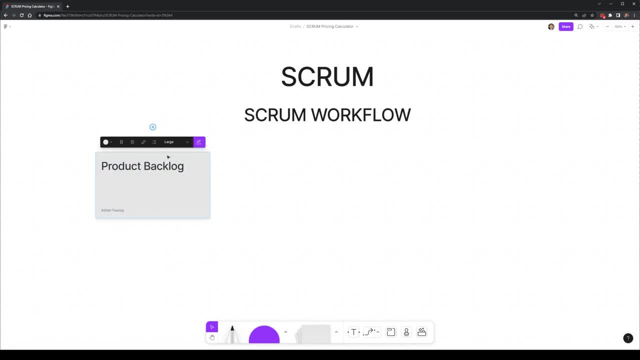 planning to do. There are a few elements to the Scrum workflow, So let's take a look at them. The very first is the product backlog. The second is the sprint Planning. Next you have the sprint backlog, then the sprint and the potential product And finally, 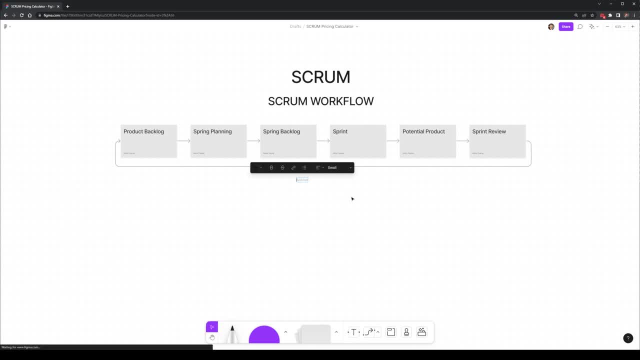 you do a sprint review. Now it's fine if you don't understand what these things are, We'll get into these, but the end process should be between one to two weeks whenever you're doing a sprint like this, But sometimes they can also last one to four weeks as well. So let's actually dig into what 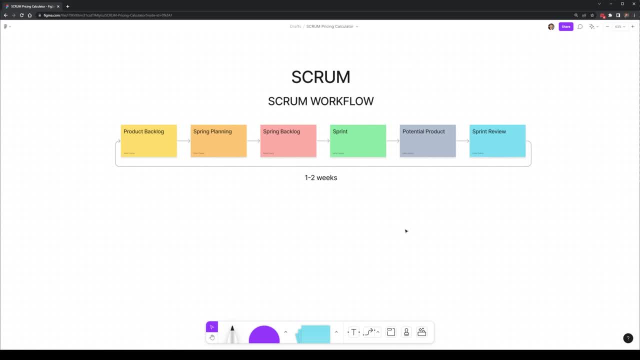 each one of these are and how they work, because they make up the essence of the Scrum workflow and all of them work a little bit different. First thing that we'll need to know is that there are three different roles when we're doing Scrum. The very first role is the one for the product owner. This is the person. 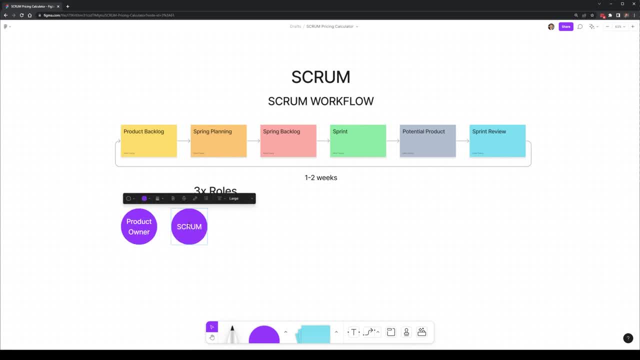 who is creating it? Maybe the company, maybe the organization, maybe the idea holder themselves. The next is the Scrum master. This is someone to help you organize and manage your Scrum sessions. They might not be a product owner, They might not be a developer. Usually there's 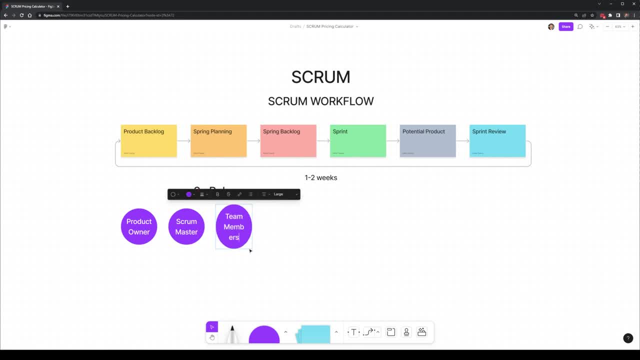 someone in between that can sort of work as a middle person and basically communicate everything that's happening. And finally you have the team members themselves. These are usually the designers or the developers or the people working on the actual product itself. It's important to define the different. 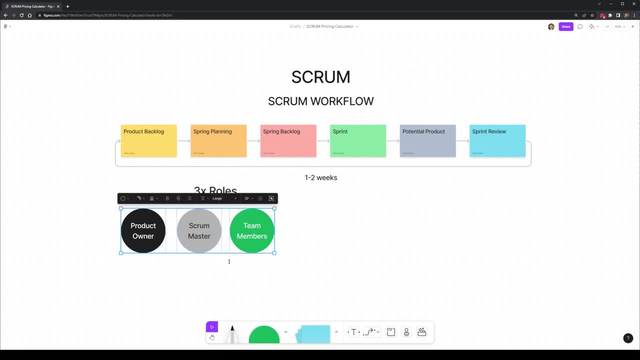 types of roles here, because some will attend certain aspects of Scrum, while others you'll want to avoid having in certain meetings, And I'll get into this a little bit later, But for the time being, just be aware of these three roles. The next thing we want to take a look at is the three artifacts of Scrum. These are something 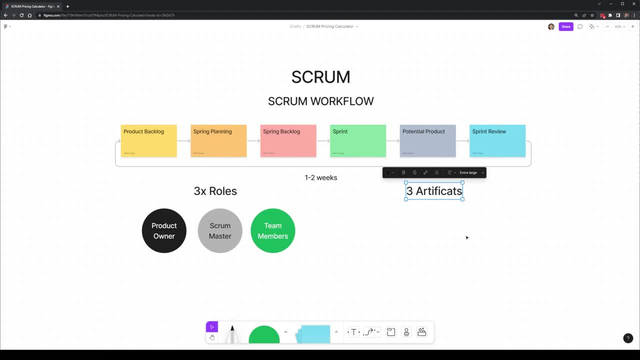 a little bit different. So let me get into exactly what an artifact is and why it's a part of Scrum. Now, the very first type of artifact is the actual product backlog, The next is the sprint backlog And finally we have the burnout chart. Now the product backlog is sort of like the features of the. 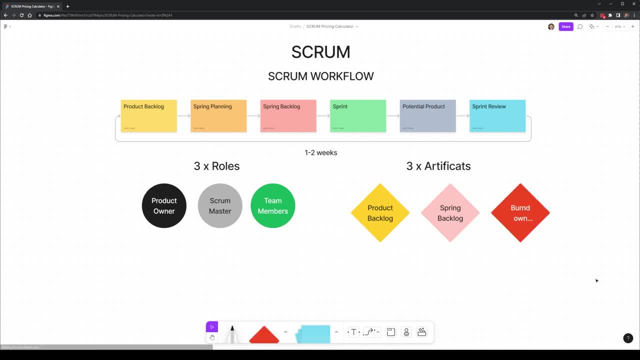 products, things like logins or admin dashboards or anything like that. The sprint backlog is sort of turning these features into user stories that can be developed, And the burn down chart is where we have a look at all the user stories and then have 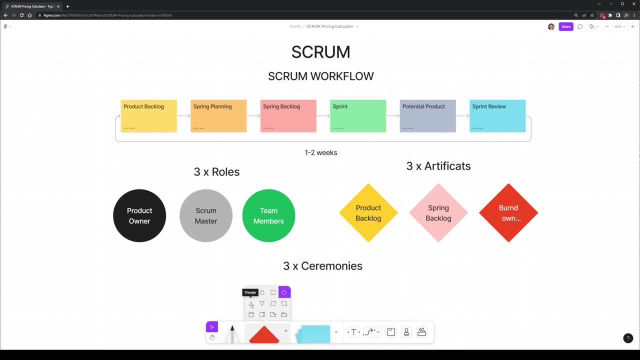 a look at how many are complete, how many are left to do, and gives you an indication of how long it'll take to complete the project. Now let's move on to ceremonies. These are basically like events that are happening in Scrum, And there are three main types. The very first is the sprint planning. This is 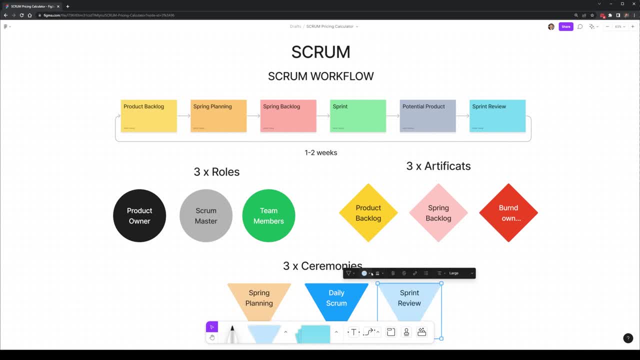 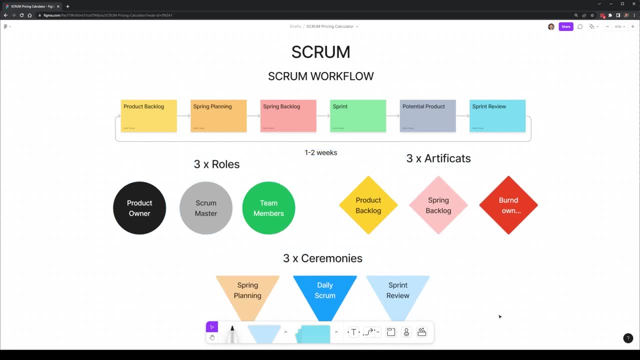 where you plan the project sprint for the one to four weeks. The next is the daily Scrum defining what has been done so far, And the final one is the sprint review, which you do at the very end of a sprint to have a look if everything that we planned was completed. 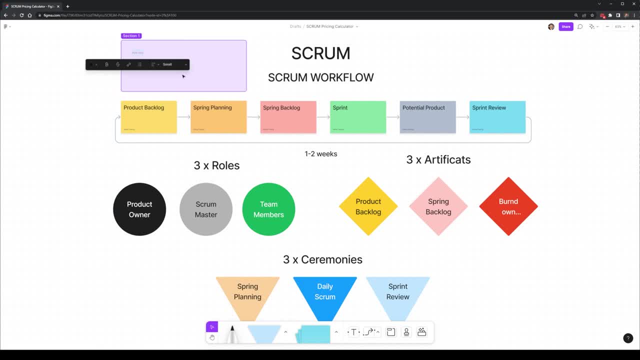 There are also a few terms and definitions that we'll be using inside of Scrum, So let's have a look at defining these so that you have a better idea of what they are and what they do. The first, most important, is the definition of done. This is an important one because 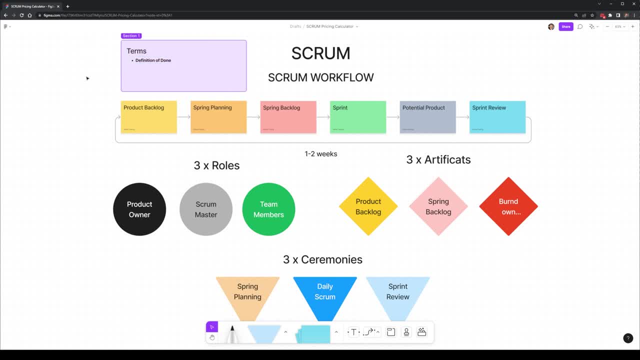 this is basically the definition of when a story has been completed. There's also the term water flow, something I'll get into a little bit later, But traditional waterfall is basically like the old way of doing projects, as opposed to using Scrum. Next, we have stand up, which is part of ceremonies, and talking about how you do your meetings. 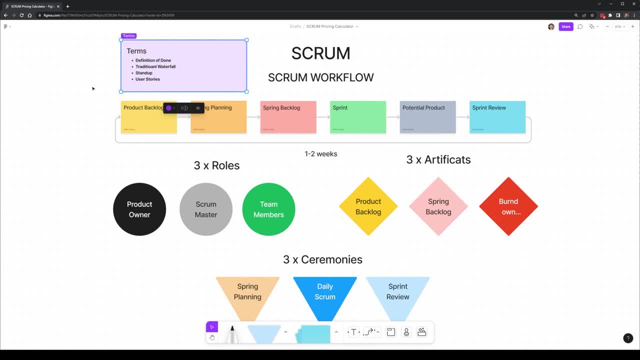 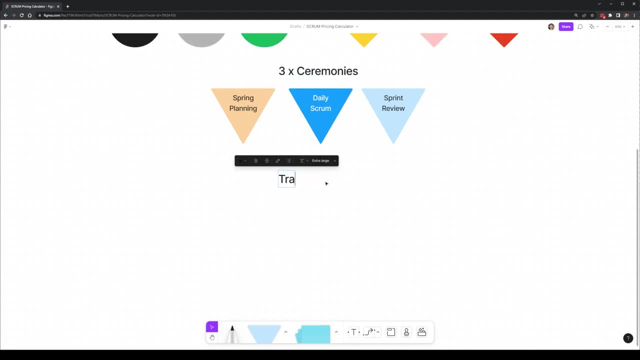 And we also have user stories. This is probably a very important one, where it basically defines how a feature is to be implemented in a Scrum methodology. So let's jump in and have a look at traditional water flow development as opposed to Scrum development. 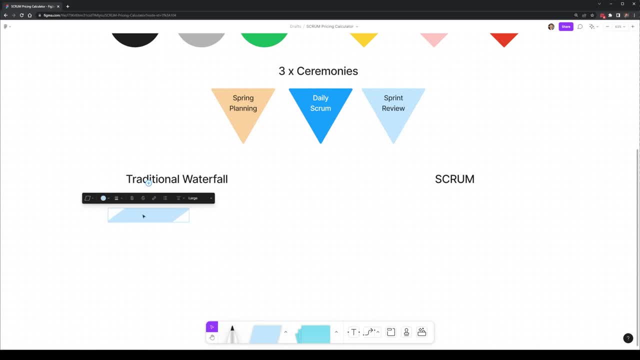 These are two very similar yet different ways of creating a project. If you've done traditional development in software, you have probably been using the water flow method without even realizing it. This is where significant time and effort is spent into building a project in several phases. The first phase is usually the planning phase, where we create the plan. 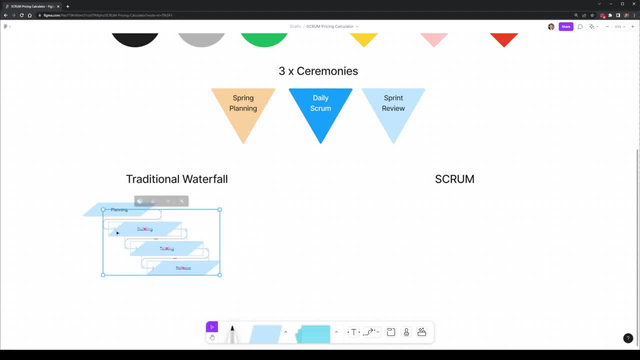 and overall objective for a project, Then we build the project and finally we test and release it. Now all of these steps happen sequentially and they can happen over a long period of time, sometimes over three to six months, And in software development that can be very long. 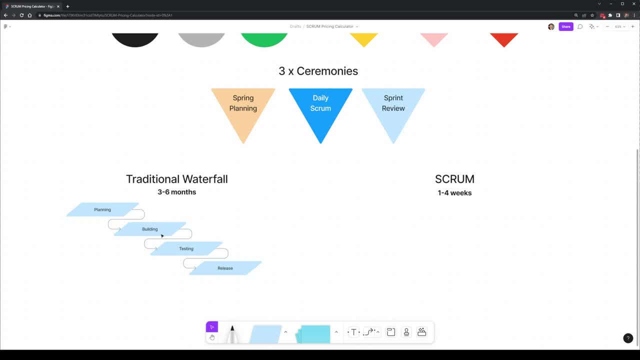 This is where Scrum basically flips this on its head, turning this sort of a structure into a one to four week structure in small units. So instead all these elements here overlap into what we call a sprint. Instead of trying to complete an entire project, just the core aspects. 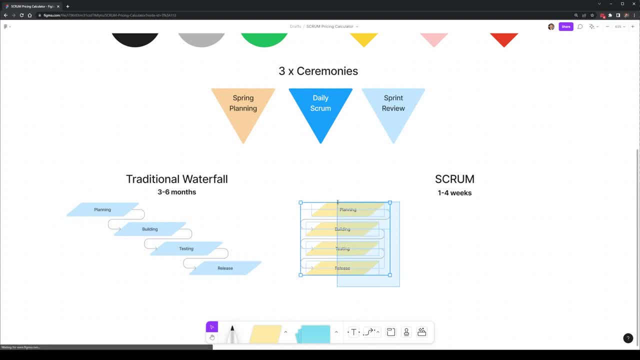 of a project, whether it would be an MVP or a product, is implemented in these steps, which we'll be having a look at very shortly- But this sprint is then done continuously so that if we need to change the project at any point in time, if there are any failures, they can be identified. 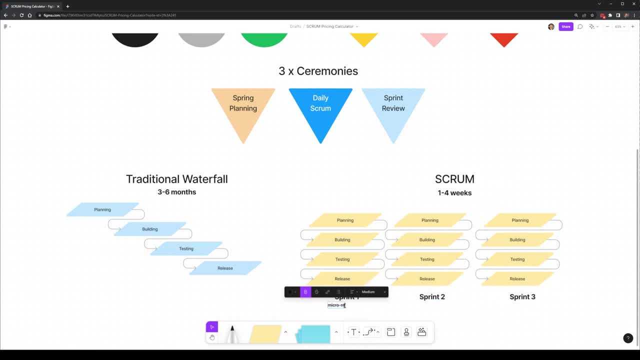 very early on, And this allows you to pivot a project or change it or modify it, depending on how you need These. micro releases are a variation of what we would normally do as a macro release in traditional Waterflow. This is a very important part of the project. because it's a very important part of the project. 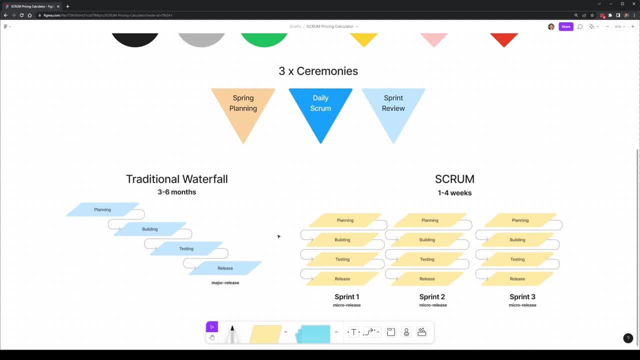 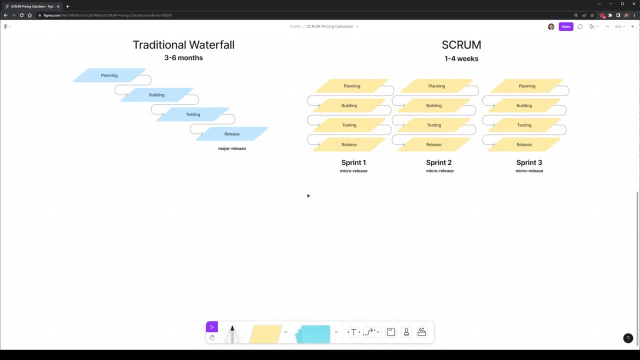 This is just a brief idea of the differences between the two types of project methodologies, but hopefully it gives you a small insight into what we'll be looking at next, which is what a traditional sprint looks like and how we create one. So let's take a look at that. 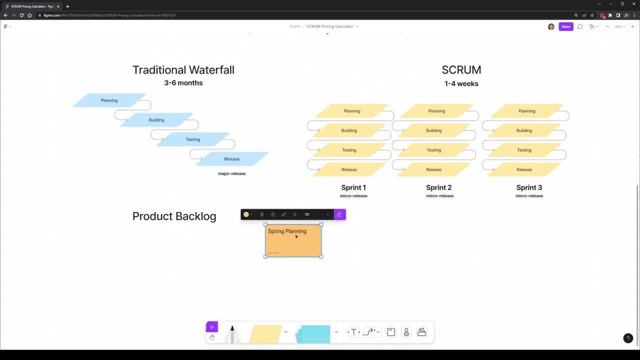 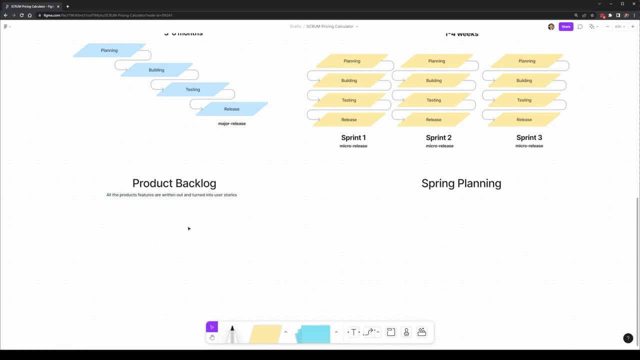 now In Scrum, the first thing you want to do is create a project backlog and then a sprint planning session. Now for the project backlog. this is where you write out all the project features that need to be implemented. You'll want to turn these into. 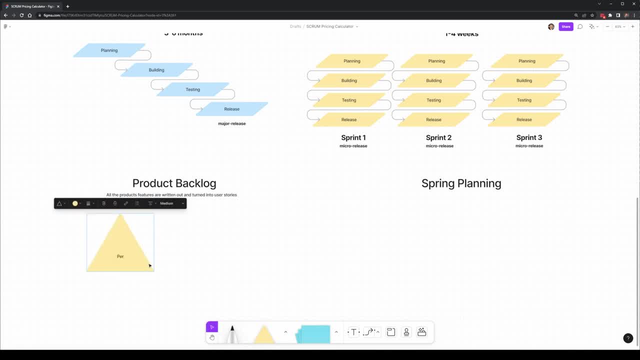 user stories And this way you'll be able to essentially create a map of all the different tasks that need to be done. This is why it's called a project backlog. So, for example, a login feature could have a number of user stories. For these, you have a certain syntax you need to. 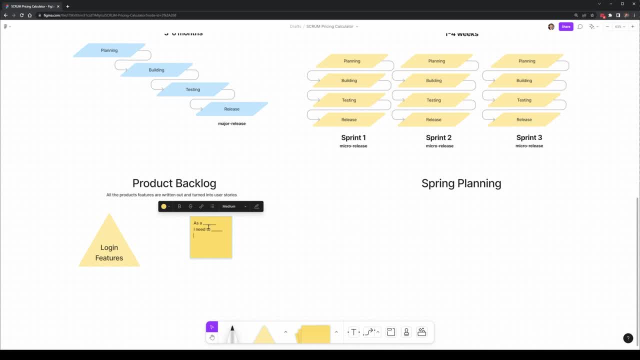 follow. Now this syntax is: as a blank, I need to blank, so that blank- You need to fill in the blanks in this type of form, And then you need to fill in the blanks in this form, And then you need to fill in the blanks in this form. 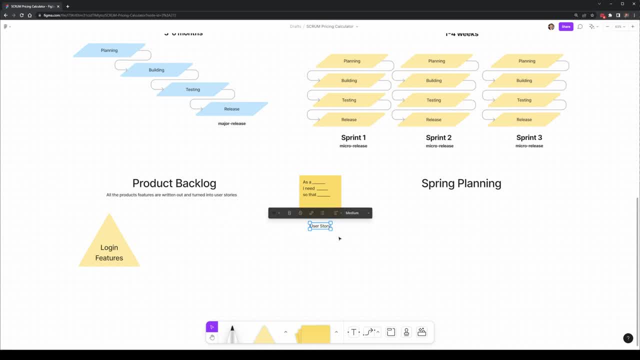 And then you need to fill in the blanks in this format to have a very well-defined user story based on what you're trying to implement. This user story can be considered here for this login features. as a user or as a general user, I need to log in so that I can access the website's backend. 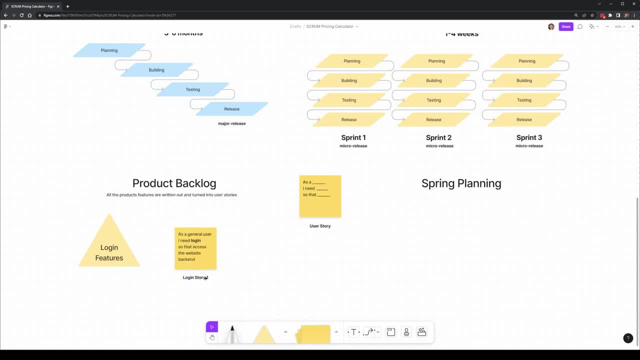 This is an example of a login story for a user. as part of the login features, A login might also have a number of user stories. So for this login feature we might have a forgotten password story. In this case a general user would say as a general user. 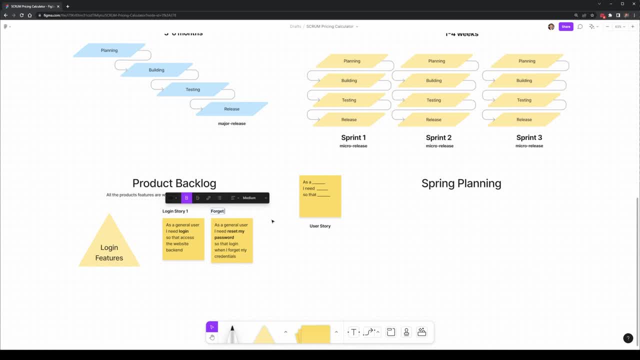 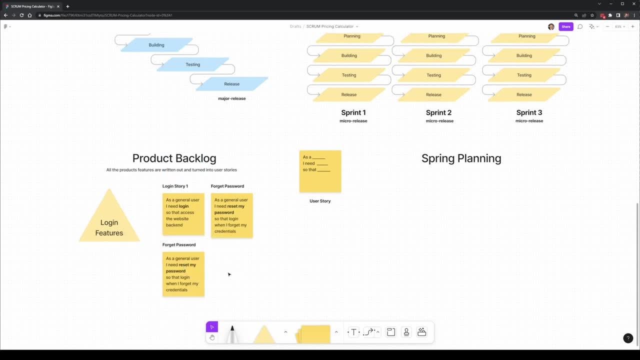 I need to reset my password so that I can still log in if I forget my credentials. Now, these are just two examples of user stories. You could have quite a few, depending on the feature that you're building out. Normally, you want to connect them, so you understand exactly. 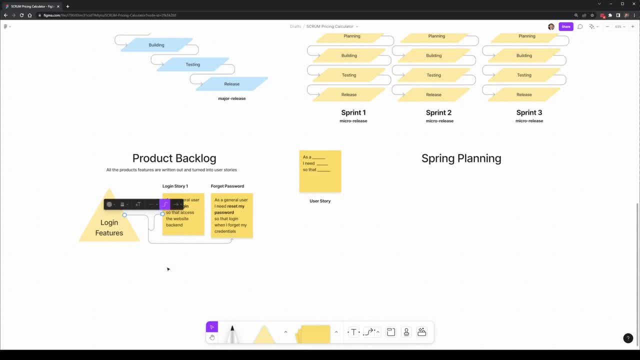 what you're building, who for and why. But once you do this, you have a nice product backlog for your scrum board that you can start using. So this is a nice product backlog for your scrum board that you can start using. 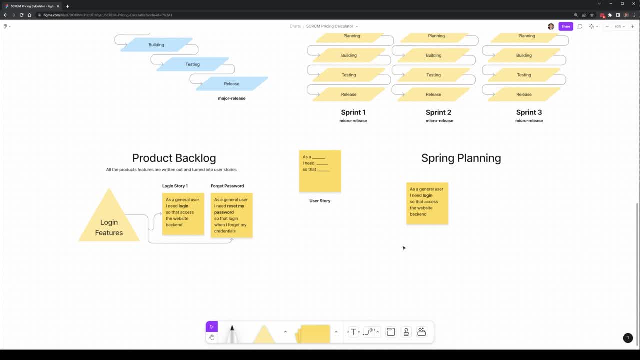 that you can start using as part of the sprint planning. Now, the sprint planning is a little bit different. This is where you start taking in multiple project backlog scopes and creating more or less a priority list of what you need to do. So if we were, for example, 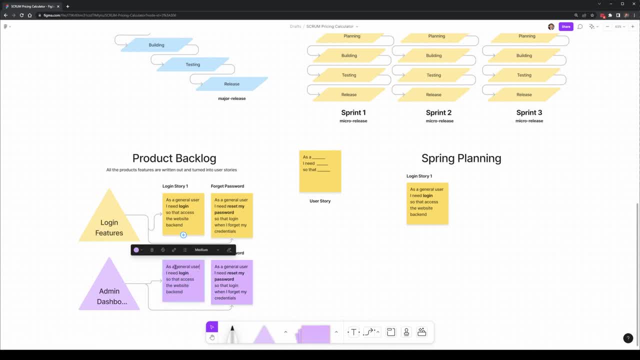 filling out this product backlog inside of scrum, we would have basically the entire product and all its features are listed out as deliverables that need to be attended And these would all be created into user stories. This way you can drag the user stories across to the 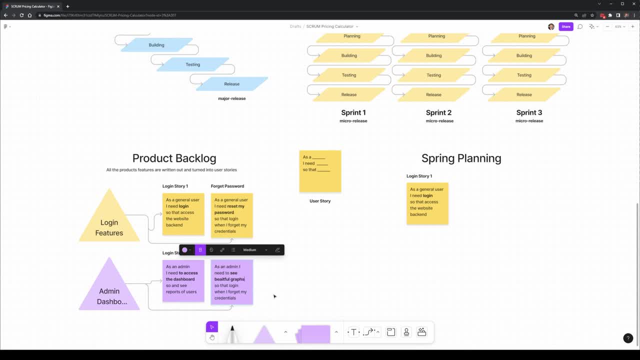 sprint planning to identify exactly what you're building. So another example of a product backlog feature here would be an admin dashboard. So the user story might go something like: as an administrator, I need to access the dashboard to view reports on users. Another: 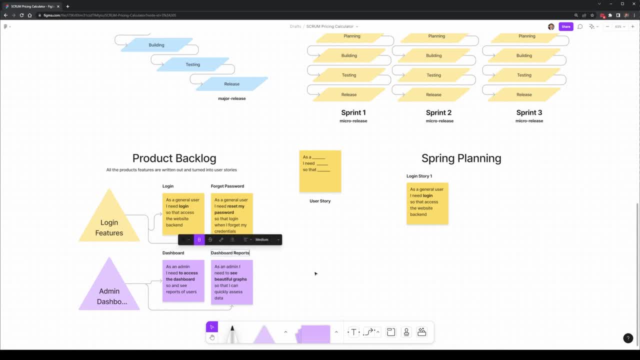 could be maybe something which is less important, such as reporting. So, as an admin, I need to have some beautiful graphics, with maybe bar graphs, in order to quickly access and understand the data. Now, when we move on to sprint planning, this is where we basically rank the most important. 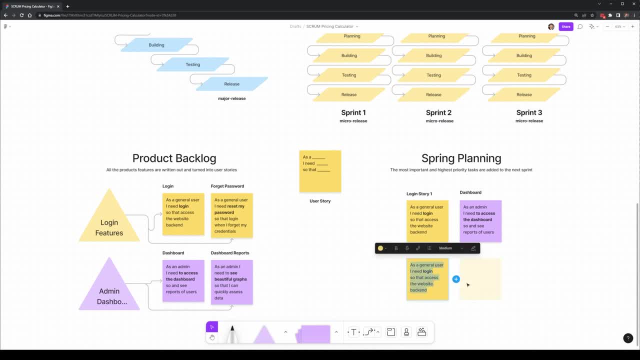 and high priority items to be added to sprints. In the terms of a login, being able to login is more important than being able to reset a password, Or for the admin dashboard, being able to access it is more important than having maybe some beautiful graphics or statistics. 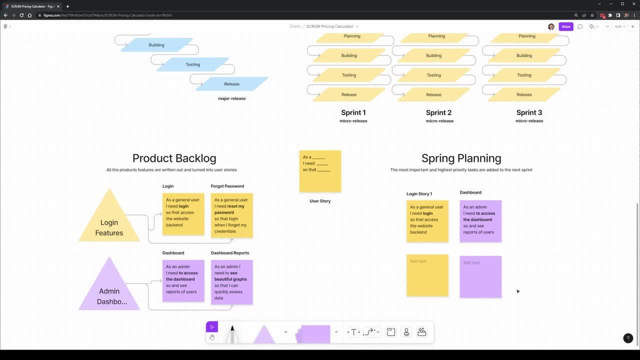 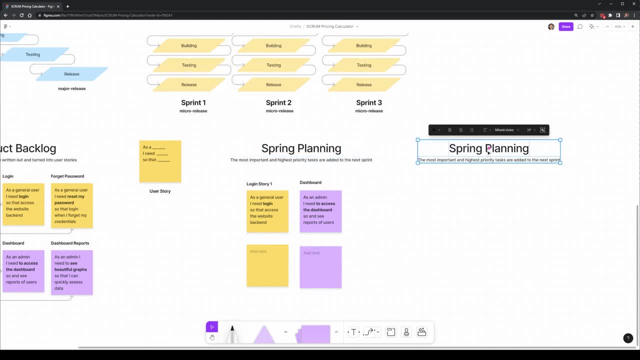 So sprint planning is basically encapsulating the most important aspects here, And once we have this, we can start arranging what the plan is for the sprint ahead. Now, the sprint ahead is normally performed when you do a sprint backlog. This is where if, for example, you've already completed 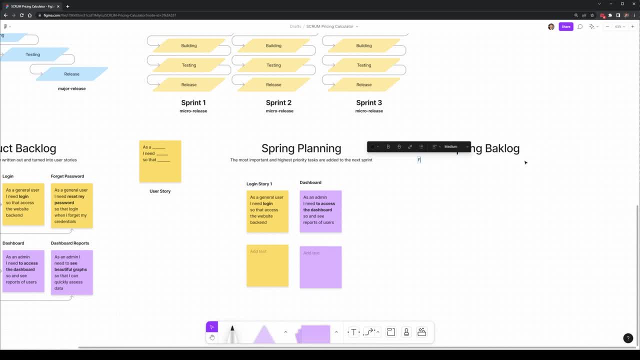 a sprint or you have one upcoming, you take a look at the objectives that need to be done, such as if there was anything missing in the previous sprint and just how much you can complete in a single sprint during the week. So that's a very important aspect of sprint planning. So sprint planning is. 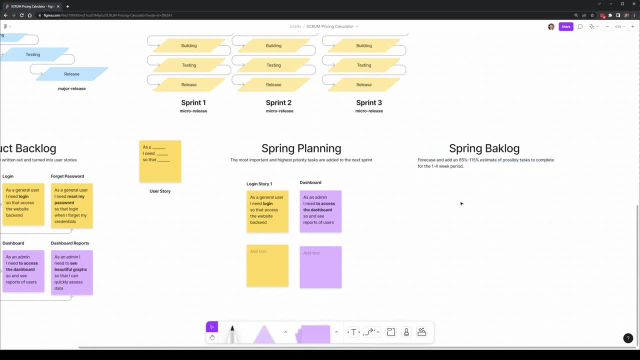 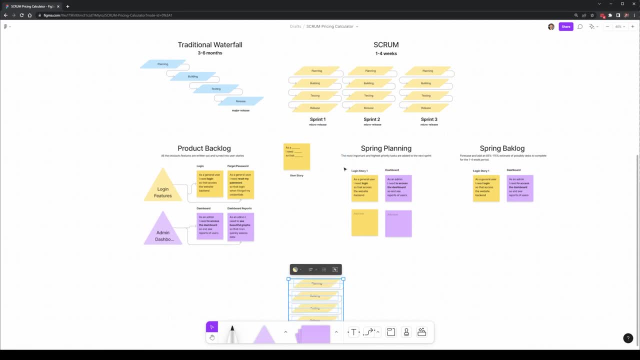 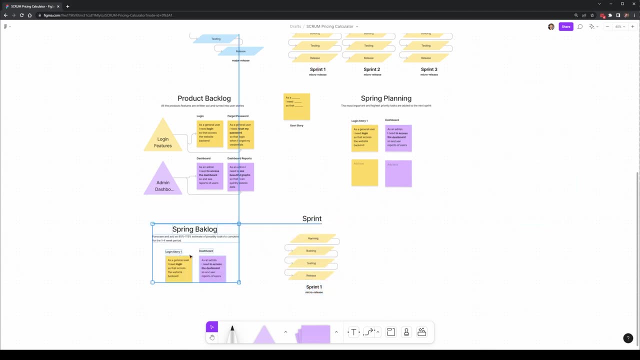 one to two week period. A good rule of thumb is often to take on board only 85 to 115 percent of how much work you actually think you can complete in a sprint backlog. So now that we have all the essentials, we can now perform a sprint. We would utilize this sprint backlog as the plan for the 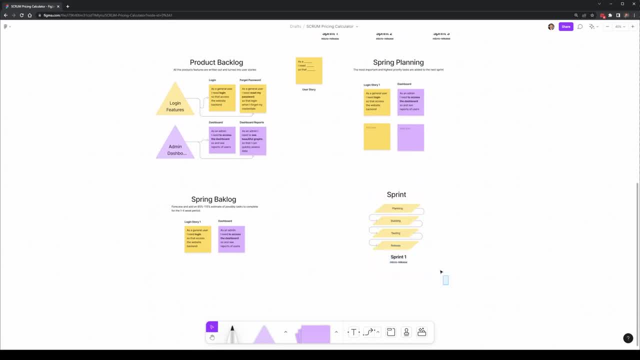 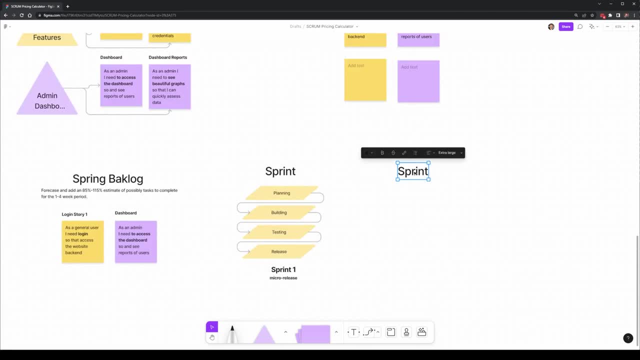 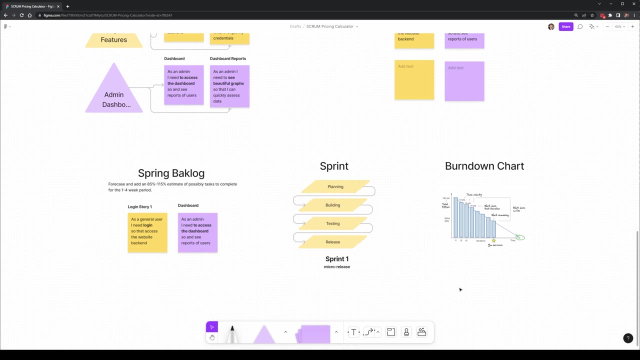 sprint and here we would complete the sprint in a quick number of phases where we're doing all the planning, building, testing and deployment of the features based on those user stories. Once we complete that, we update a burndown chart. This is a chart of the entire product backlog as well as. 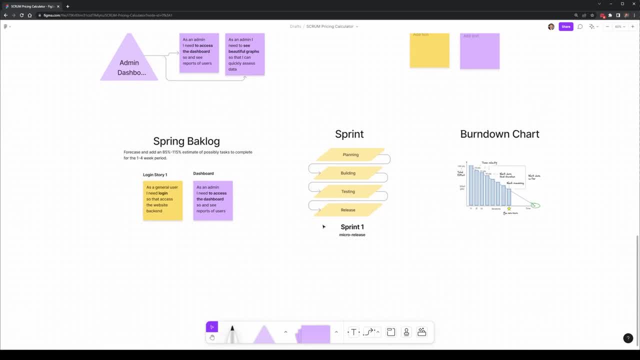 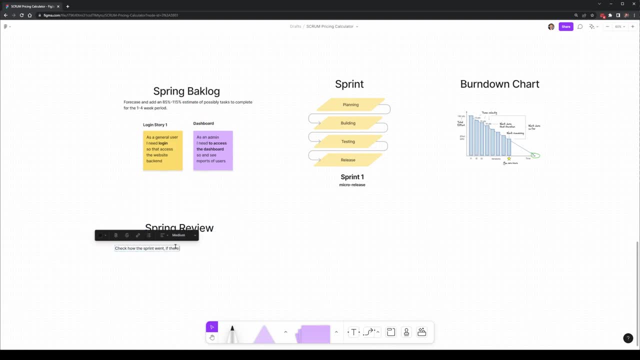 all the tasks that have been completed so far to give you a graphical representation of how the progress of the project is going, how many user stories are left and when the estimated time for the product will be complete. Now we can move on to a sprint review. Having completed a sprint and 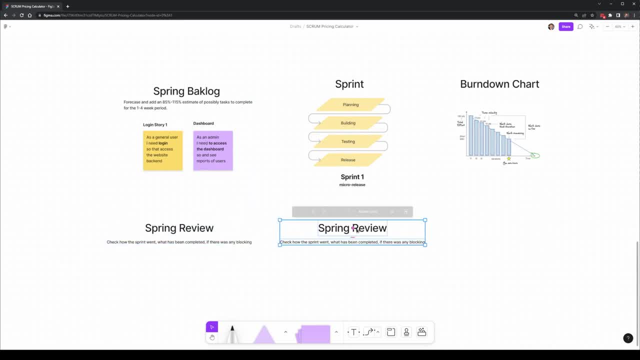 finishing the task involved. basically, the sprint review is where the product owner, as well as the scrum master and maybe the developers, review the entire project at the end of the sprint. Now, this is different as opposed to, say, a daily scrum, which is more akin to just the team meeting up with the 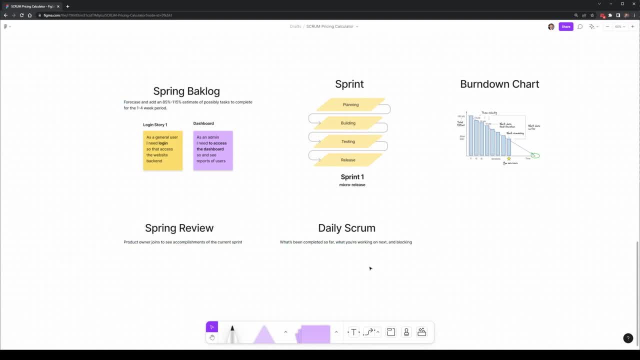 scrum, master, in order to view the progress so far on a daily basis. Normally you wouldn't have the product owner involved in the daily scrum because obviously it's not a daily scrum. So you wouldn't have the product owner involved in the daily scrum because. 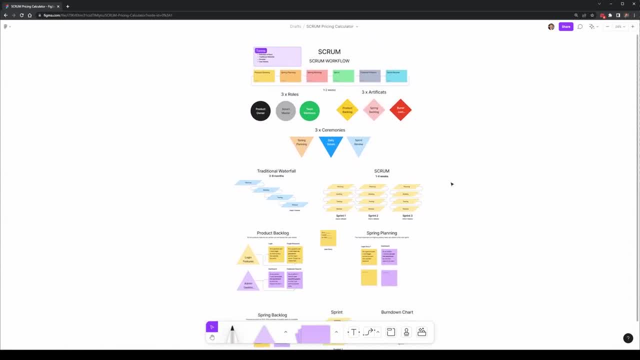 it's not a review, it's just a summary of the day. Now, all of these tasks, basically done in a sequence, and repeating, constantly encapsulate scrum and how it's used in software development. When you're coding, when you're building software, developing it, whether you're designing it. 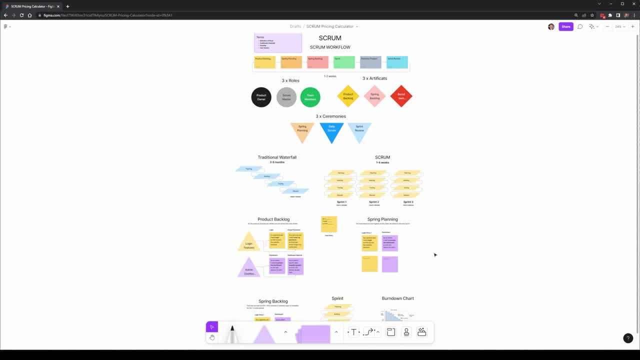 scrum can come in handy in order to help you better plan for that. One project I'm working on right now is a pricing calculator, and it's one that I'm doing inside of Editor X as well as in Nodejs, and I've got a Figma board. So let's have a look at how I can do some working on that, and then I'll 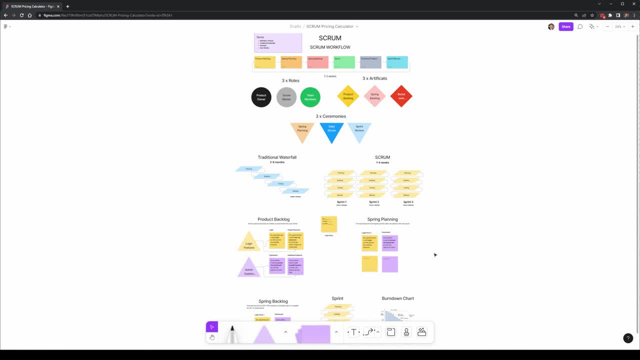 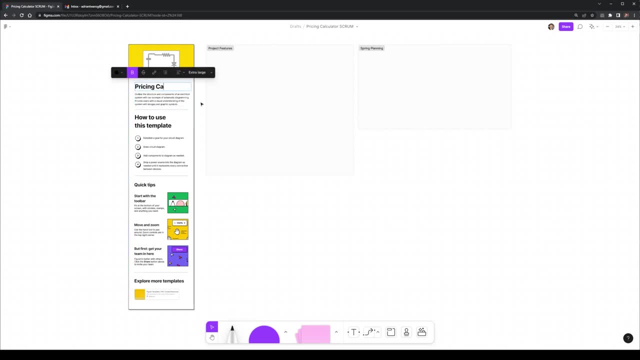 can incorporate an example of scrum so that you can actually see it in practice. So what I've got here is a brand new document and I'm going to also link this in the description below, similar to what I'm going to do with the scrum board, so that you guys can copy these at any point in time and reuse. 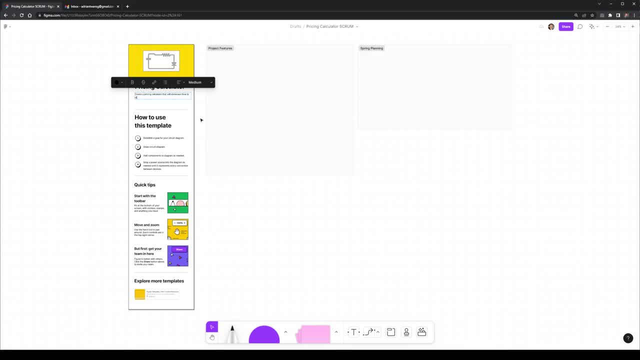 them. The first thing I want to do here is define the project For this project. here I'm creating a pricing calculator, So the definition of the project will essentially include the fact that I want to create three or four different types of pricing calculators where people can, for example, 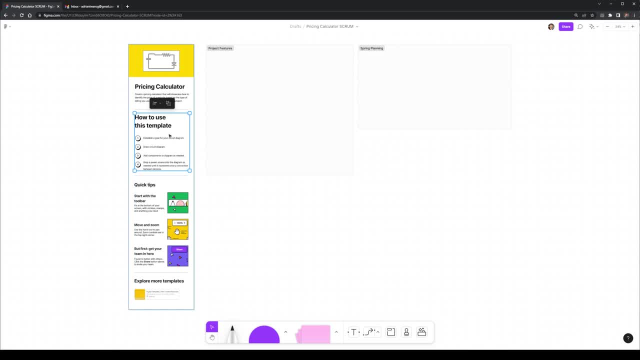 put in whether they do hourly, fixed or even value-based pricing and utilize this calculator to define the price that a website might cost. Let's figure out the scrum template here of how we'll be doing this systematically. The very first thing we want to do is create the project features. 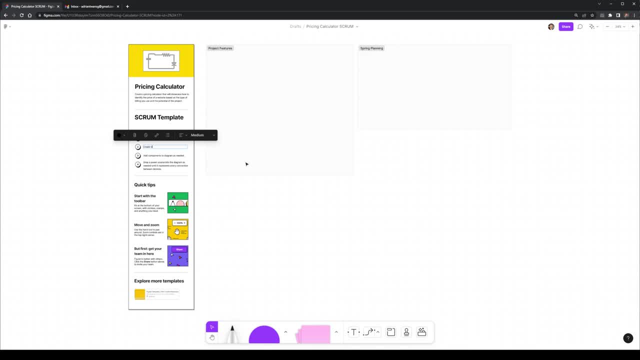 These are the features that will make the project possible. So these will be like creating the calculator itself or having the page that we're going to use to create the project. So I'm going to create a page in Figma or in Editor X. The next thing we want to do is create a sprint planning. 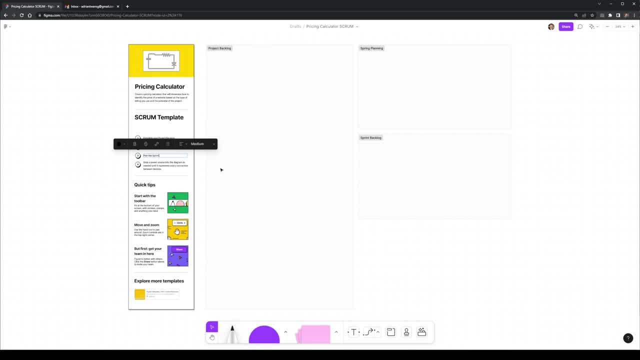 session. But before we can do that, we need to create the user stories based on the features that we're creating from the project backlog And, finally, what we're going to do is make sure to actually perform a sprint. Now, the sprint in my case will probably happen every week, but it depends. 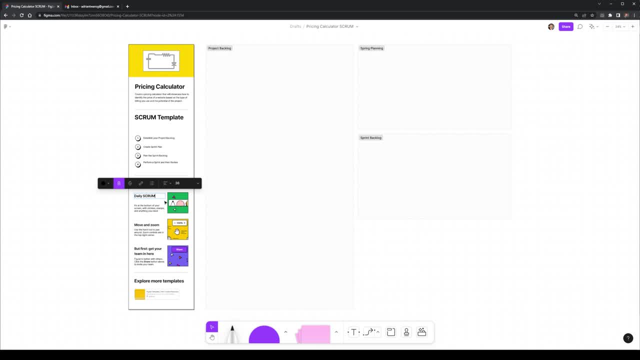 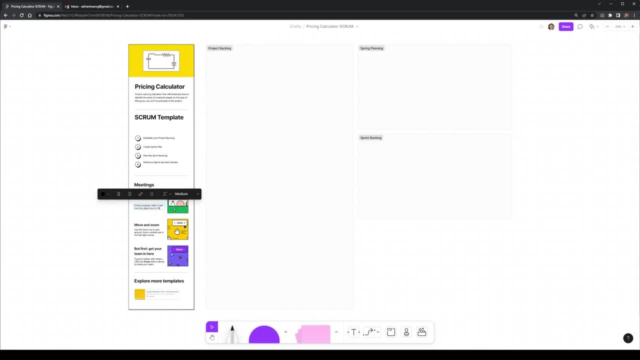 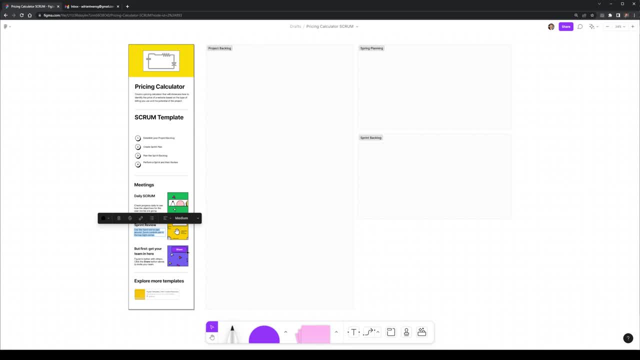 daily scrum. This is where you check in with yourself or others to basically cover the progress that you're doing. So in this case, I'll be checking in with just myself to make sure that I'm on track to building this pricing calculator. The next thing we'll need to do is a sprint planning session. 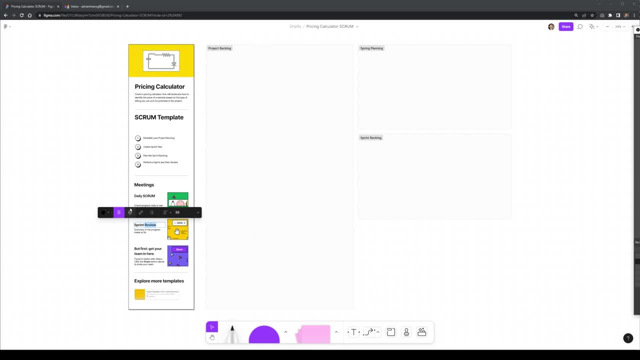 And in this session, we're going to have a look at exactly what I want to do. Of course, building a pricing calculator won't take a single week, and instead we need to define exactly what tasks want to be completed at what week. Now, right now, there'll be lots of tasks, and 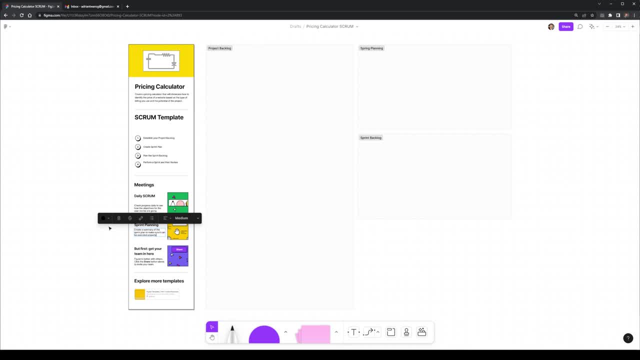 even just building out one aspect of a task might not be that simple, because a user story that might, for example, involve getting the price for an hourly based website might require a back-end API, a front-end UI and much more. The final thing here we'll create is the sprint review Now. 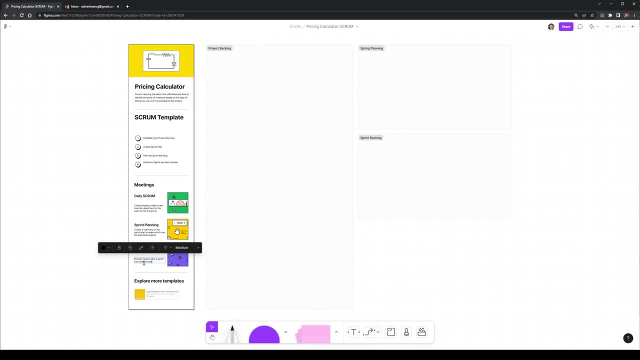 this meeting in itself is basically at the end of the session, so this could be for me, for example, at the very end of the week, where I can review exactly what I did for this sprint session, and it can also be with the project owner, which, in this case, is just me as well. Now I'm going to define how long. 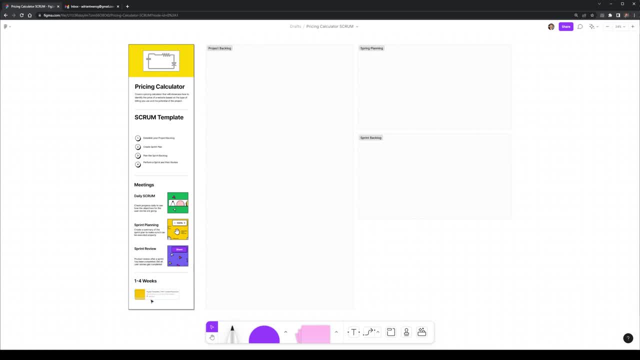 the sprint should take here at the very bottom. I'm just going to do one to four weeks, but in my case it will just be the one week. Great, so we've got all the summary here for the scrum session I want to create. Next, let me create the backlog here, the project backlog of the tasks that I want. 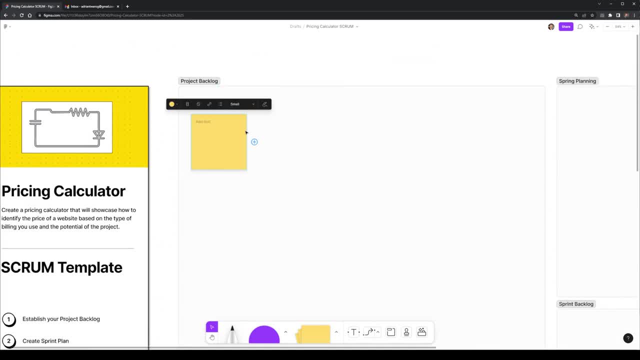 to do Now. I'm gonna try and define this project backlog with sort of the features I want to complete and in this case there are three main features and these are the types of pricing calculations I want. The very first is the pricing based calculation, the second is the fixed based. 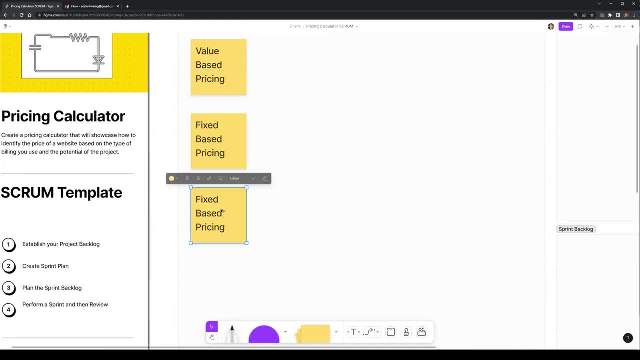 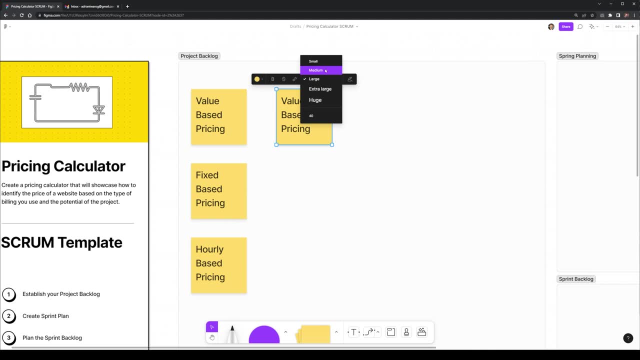 pricing. and the final one is the hourly based pricing. But before we get into that, I want to make sure that I have a general application that works. I also need some micro tasks, because these are sort of very high-end project features, and here is where I can start creating some stories. 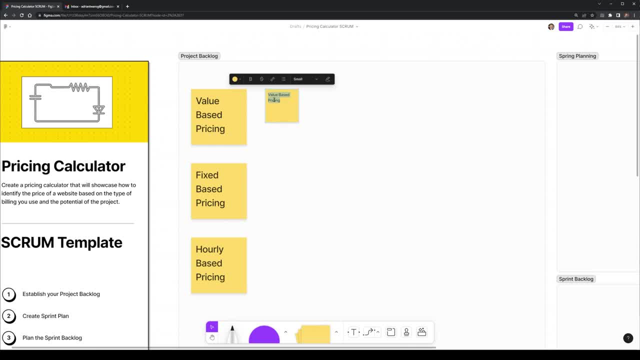 based on these features, These user stories. I'll be dragging along to the sprints later on. so let's define these really clearly. I'm gonna give each one a bit of a title so that we can reference it properly, and I'm also going to put in a title so that we can reference it properly, and I'm also going to 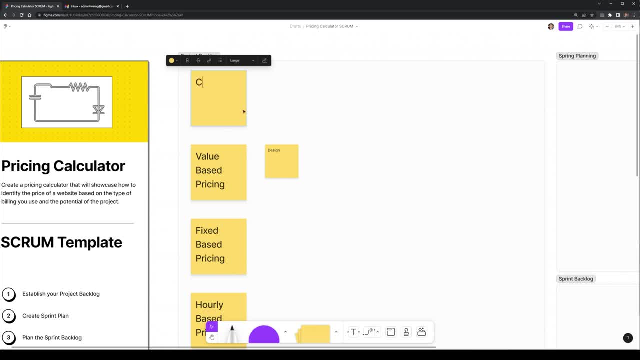 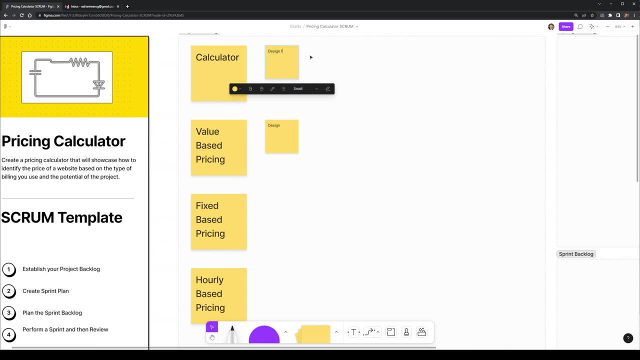 put in a title so that we can reference it properly, and I'm also going to put in a title so that we can place it in alignment with the other content that I'm creating. Let me create one here for the general calculator, because I think that also needs its own number of stories, and here I'm gonna start. 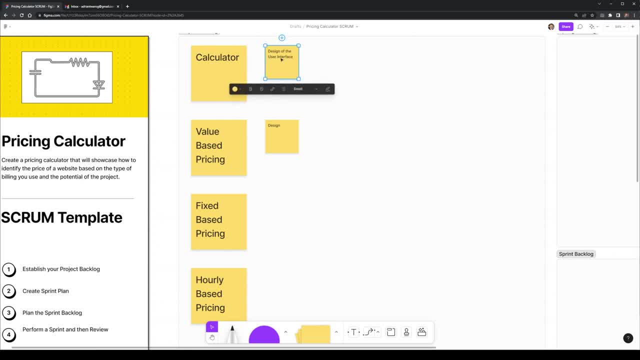 off with a design story. Now, this design story will be to basically have the user interface for the calculator, and the story will go something along the lines of: as a user, I want to see a calculator that I can use to get the pricing for a website. So here I'll define that as is. 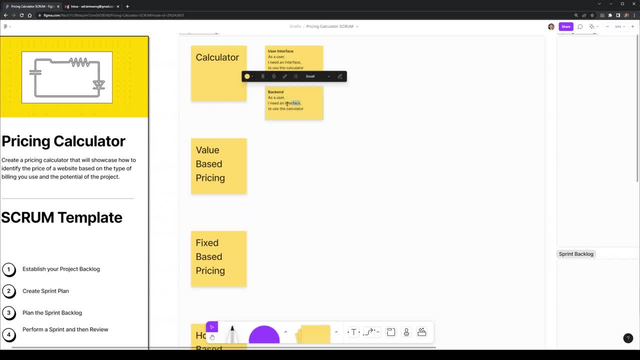 There are a heap more tasks, so let me just go through and create them right now. These will include things like creating the user interfaces, creating the functionality both on the front end and the back end, creating some of these things inside of Figma or Editor X and then putting it. 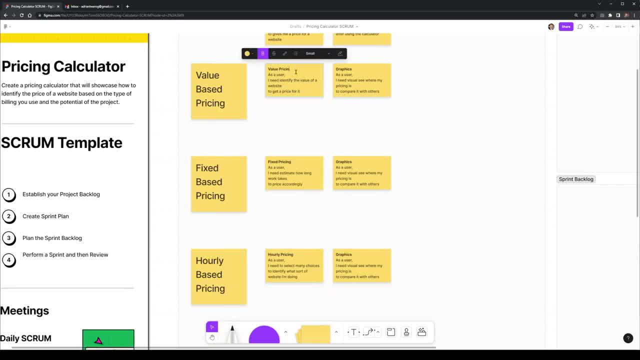 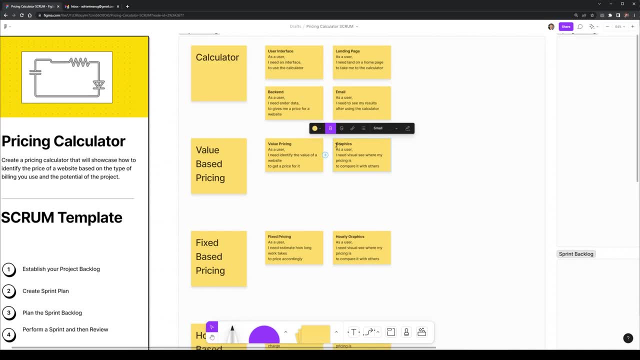 all together. The end result here is that we'll have a backlog, which basically is the entire project as it needs to be completed, which is perfect. This can be refined over and over if you really need, but normally, once you've defined this, you want to have a full project, So that's what I'm going to do here. 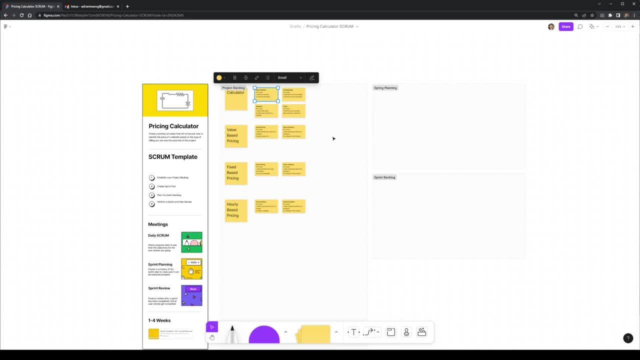 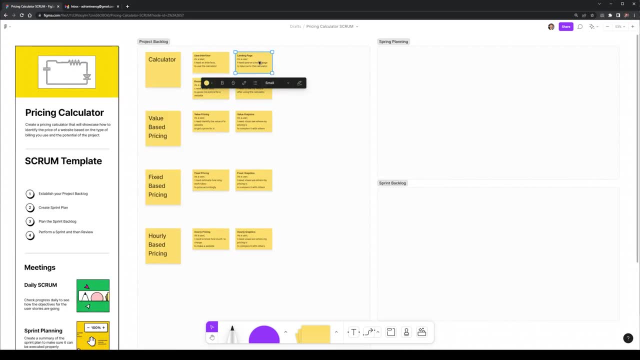 To do this. you want to keep it more or less the same. With this done, we can now look towards the sprint planning session, as well as the sprint backlog. Now the sprint planning session will involve looking at all the tasks and selecting the most important to prioritize for the sprint run. 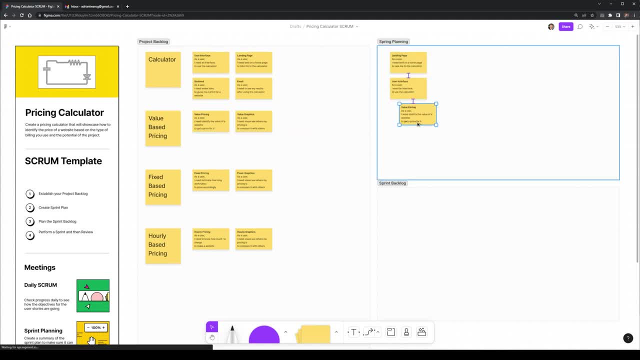 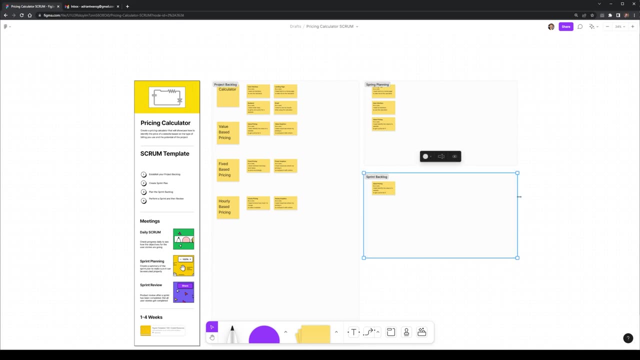 These are the tasks that I'll be doing during the week, and these are the tasks that are achievable in that week too. I just selected three main ones here, which is a little bit of UI, a little bit of pricing calculation, which is maybe hourly pricing or value-based pricing, and then I'm going to put